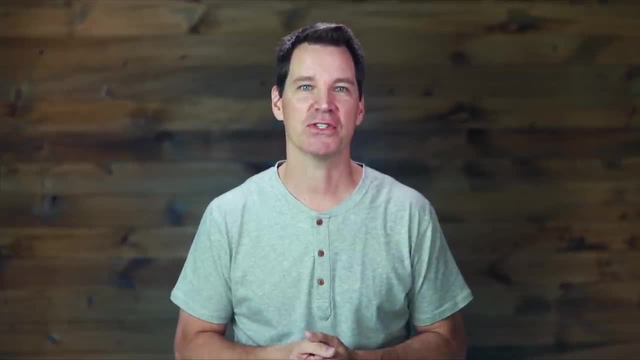 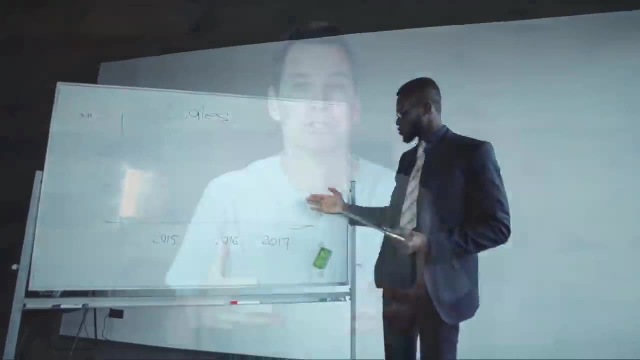 This is probably the most recognizable communication skill of all time. It could be a big presentation or speech, but it could also mean standing up to share a three-minute message in front of a small group at a meeting. It's unusual that entry-level employees are 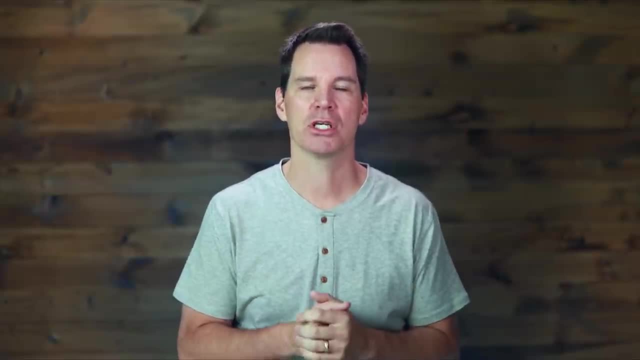 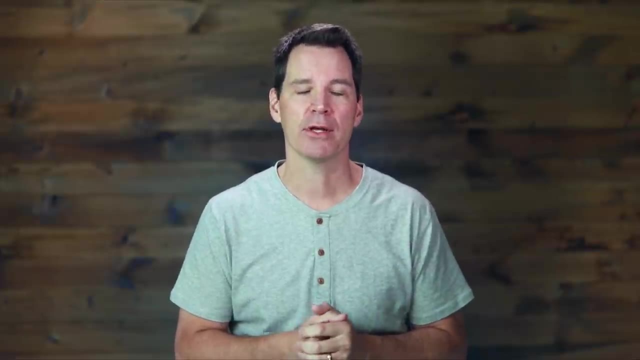 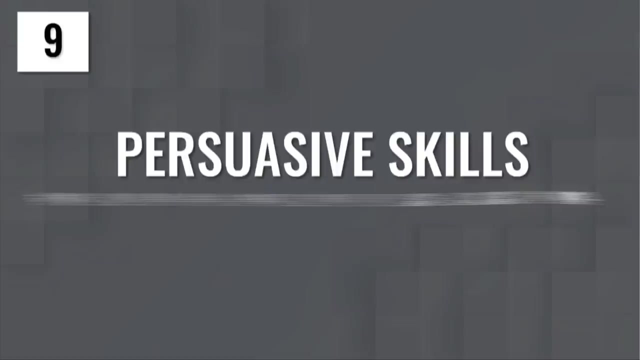 great at this unless they majored in communication in college. But on the flip side, if you are a strong stand-up speaker, you will instantly separate yourself from the crowd. People see good public speaking and they say to themselves: that's a leader. Number nine is persuasive skills. 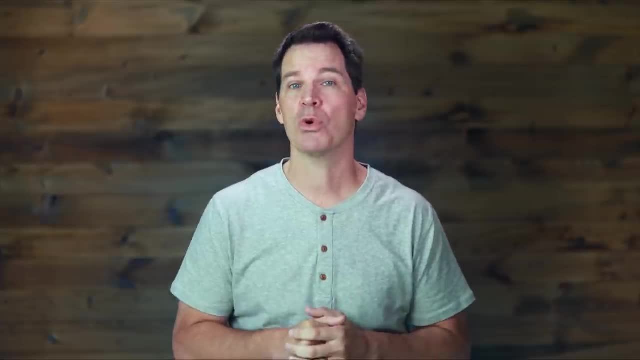 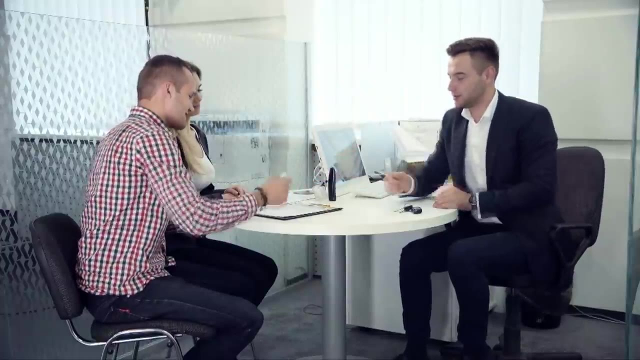 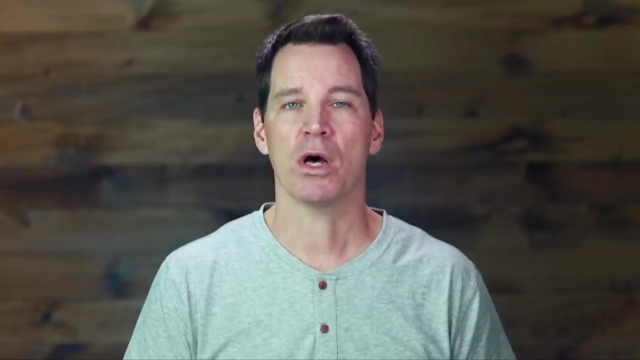 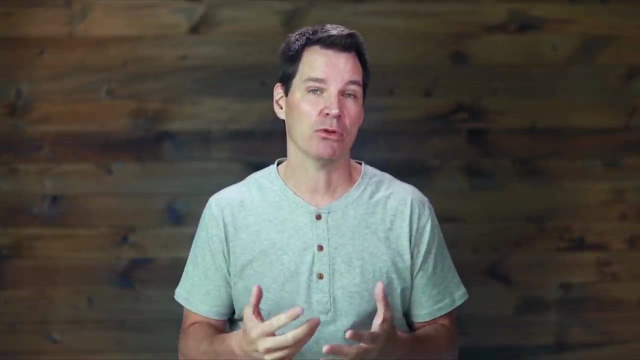 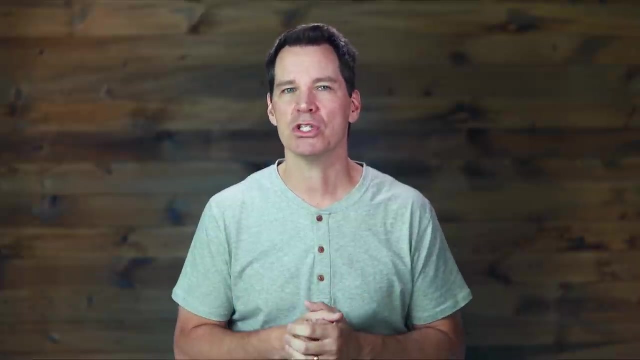 Persuasive skills are crucial because we are constantly making requests for approval and support. The most effective persuasive communication usually involves explaining to listeners that there is some need to communicate, And that's what I'm going to talk about in this video. Number eight is interpersonal skills. This is that type of one-on-one communication we do. 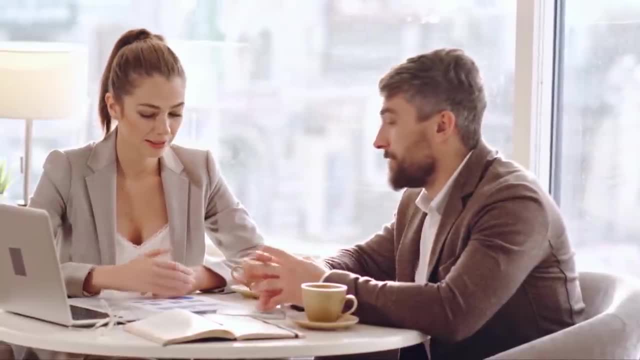 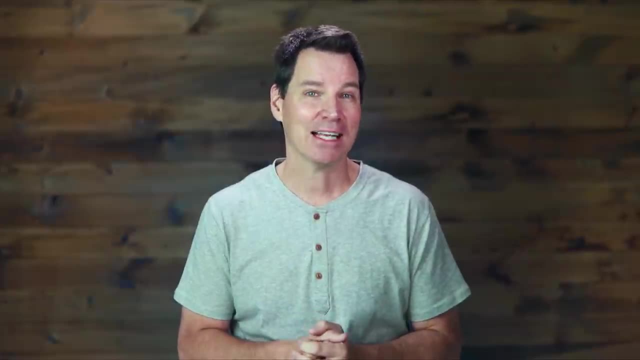 with our friends and significant others. At work. we interact one-on-one with colleagues, supervisors and subordinates. There are constant discussions about how we can communicate with each other And when we do that, we demand on task-related communication, like dealing with facts, figures and spreadsheets. 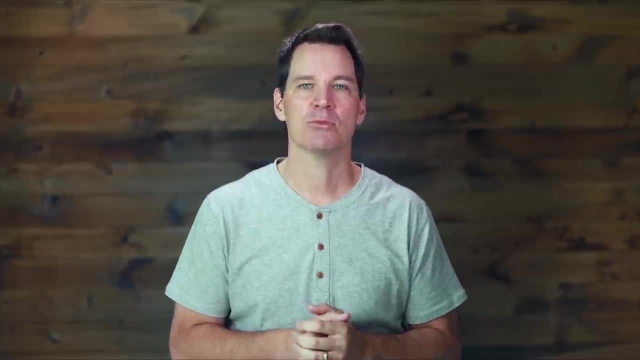 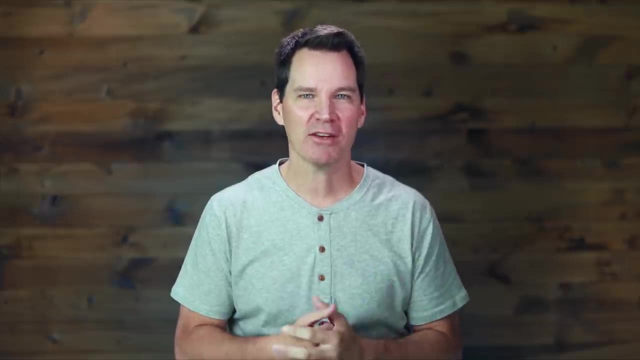 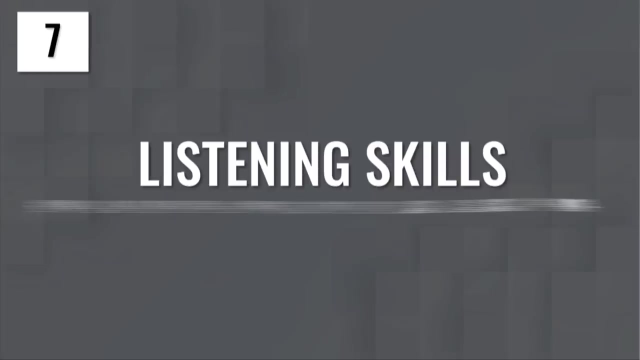 all while working under pressure. This context makes it all the more important that we take the time to also interact in supportive and respectful ways to create mutual understanding and satisfying connections. Number seven is listening skills. This is perhaps the most underrated communication skill I know of. Good listening is a hidden superpower. 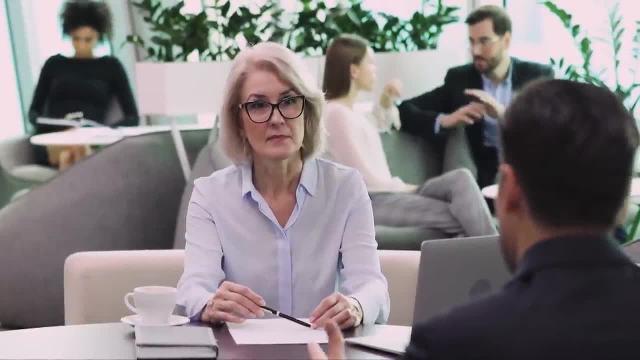 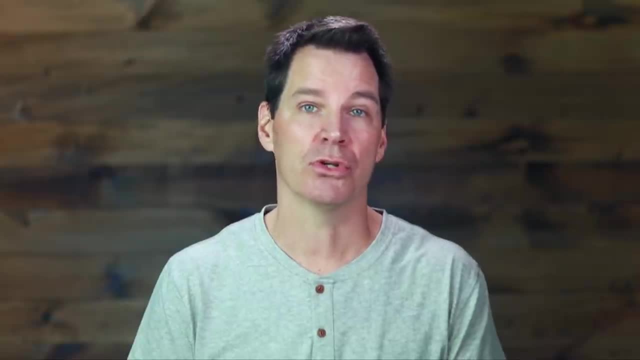 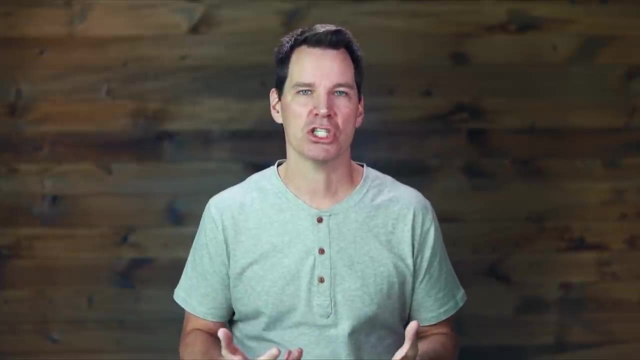 This involves removing distractions, tuning in and preparing yourself to absorb the other communicator's message. This could be listening carefully to learn a new skill or important information, or it could be listening to be a supportive ear and build genuine relationships at work. I have heard it said that good leaders are good listeners. 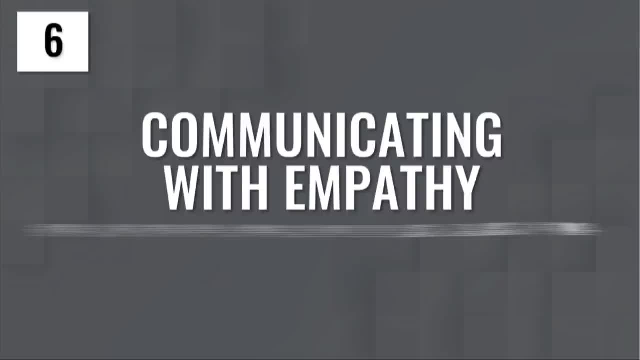 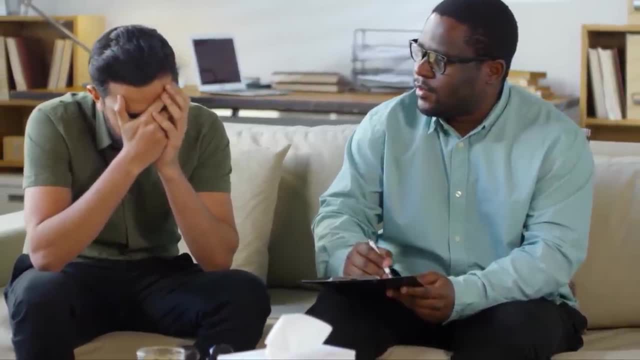 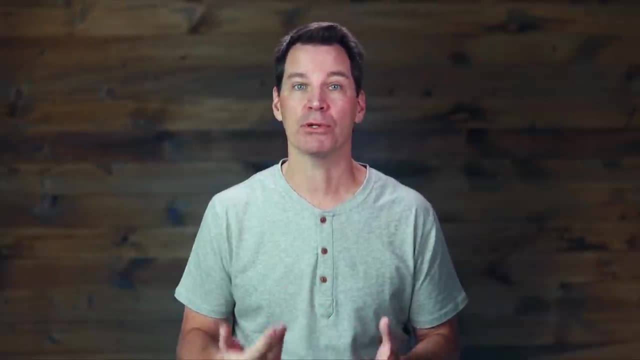 Closely related is number six: communicating with empathy. This cuts across all communication contexts. Empathy is our ability to put ourselves in the other person's shoes, to feel what they might be feeling. That empathy helps us understand where people are coming from and it builds trust. 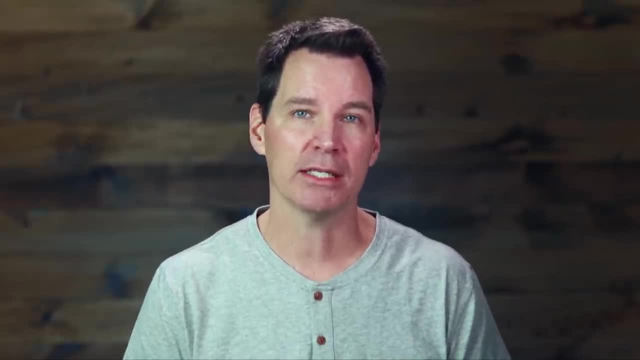 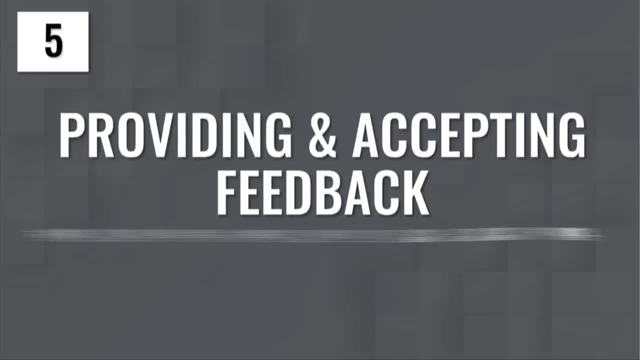 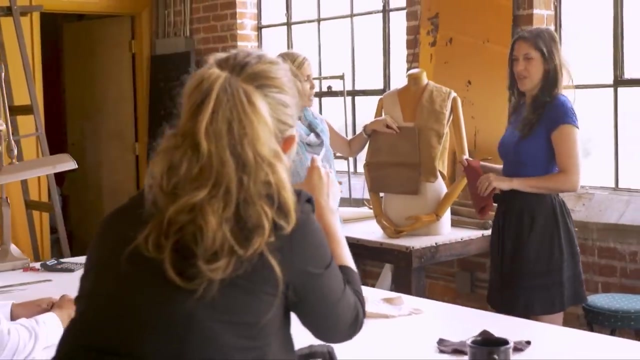 When we care and keep other people's interests in mind, we are very likely to create more helpful outcomes. Five is providing and accepting feedback. As a supervisor, you will have to provide your employees with feedback to help them develop, And we can't just point out their 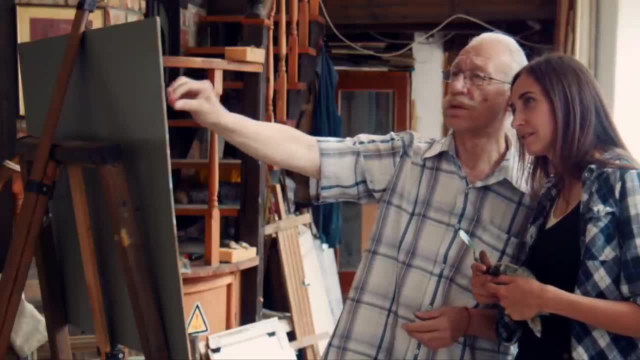 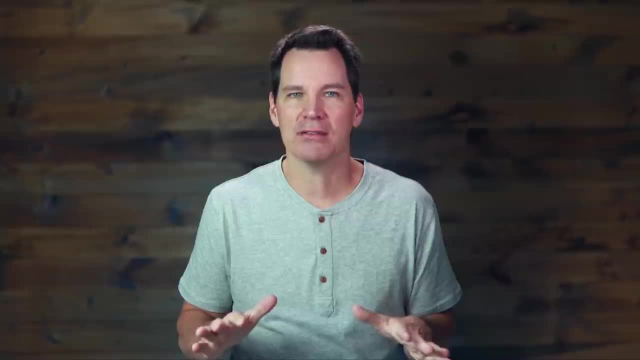 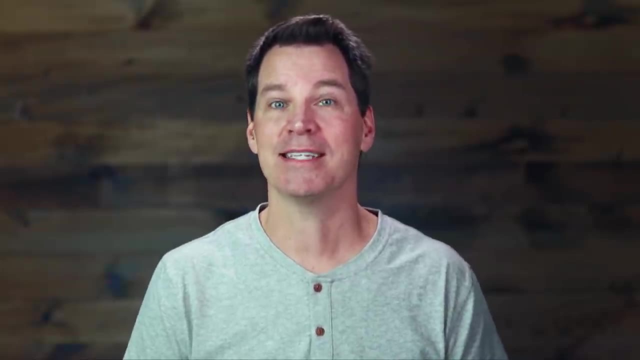 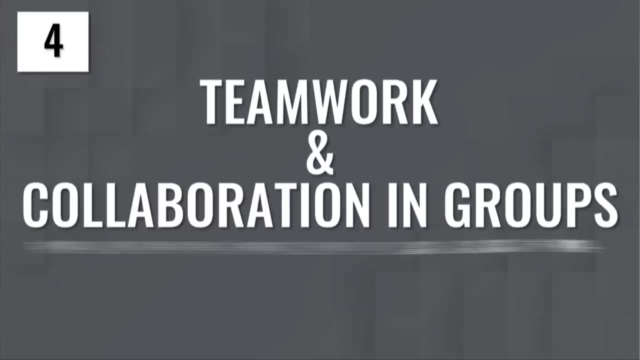 and receive feedback. It's easy to get defensive, especially when feedback is not explained in a helpful way, But if you can learn to be open to feedback and find something helpful in it, others will count it as a valuable communication skill. And fourth is teamwork and collaboration in groups. Working in teams is exponentially more. 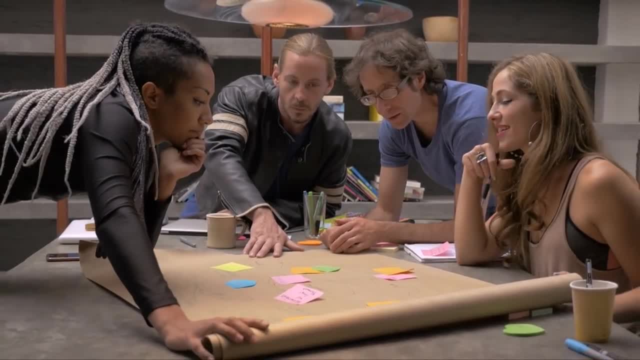 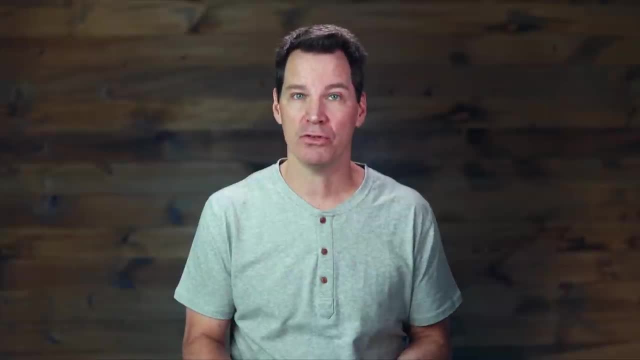 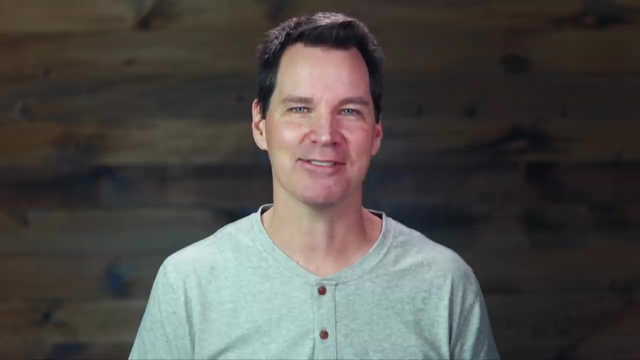 complicated than working one-on-one. People who are good in groups have good task skills like asking good questions, providing helpful information, offering a point of view, And relationship dynamics are also important, like encouraging and supporting others and staying positive. Nowadays, it's hard to picture getting promoted if we aren't good with groups and teams. 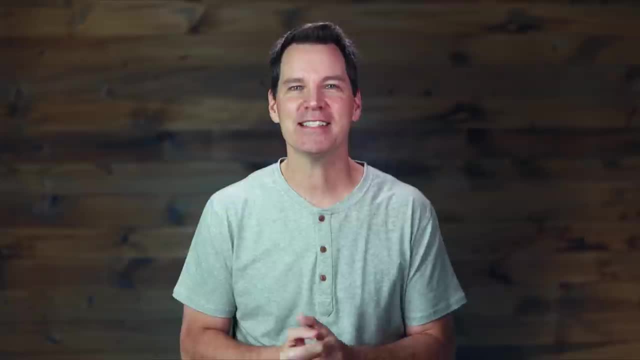 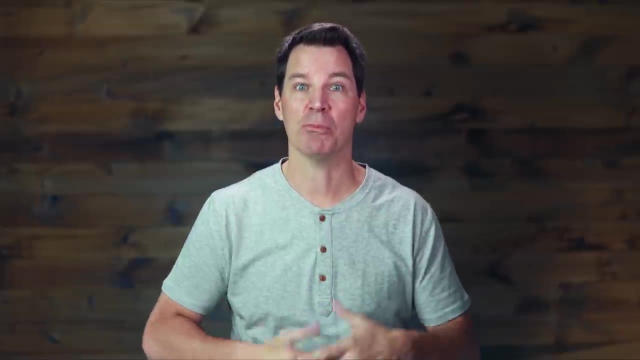 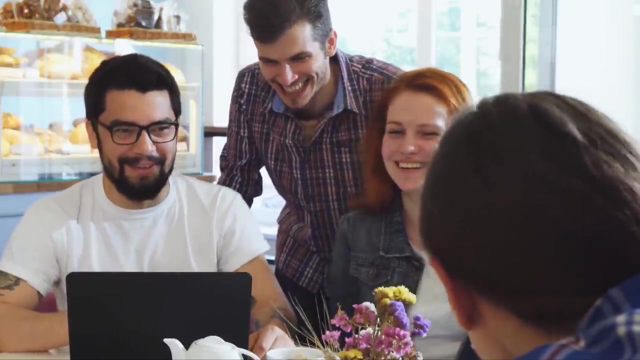 Three is nonverbal communication skills, And this isn't a separate skill. It overlaps with the others we've mentioned. Still, our nonverbal communication creates a powerful impression on others. Our nonverbals give off a vibe that shades everything we say and do. I know a guy who 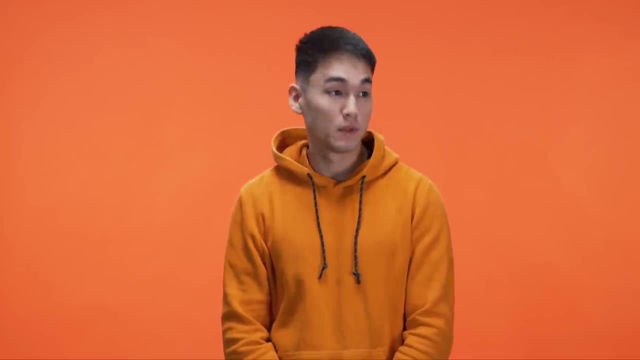 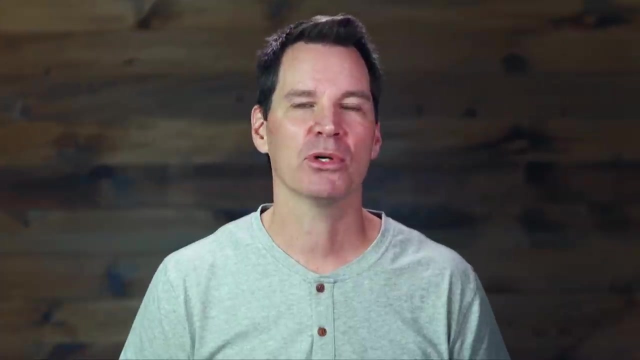 frequently rolled his eyes and made frustrated facial expressions at meetings And his supervisor finally talked to him about it and he honestly didn't even realize he was doing it. Our nonverbal communication and body language can be so automatic. But, like I said, nonverbal communication is a 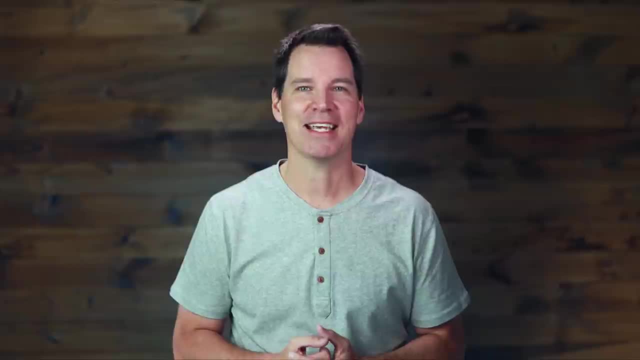 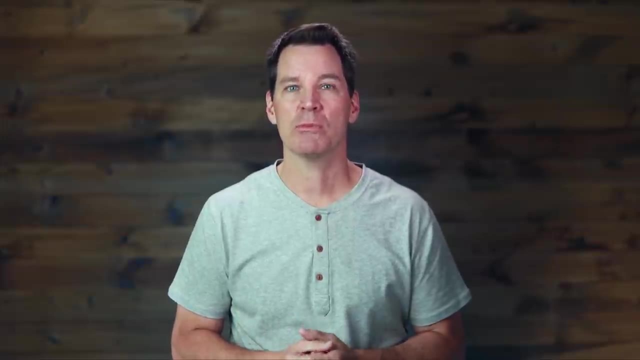 like the others on the list, we can make improvements with some self-awareness and practice. And number two is phone skills. Since we are not face-to-face on the phone, we notice other people's tone of voice and timing much more than usual. If somebody pauses for too long, it can.